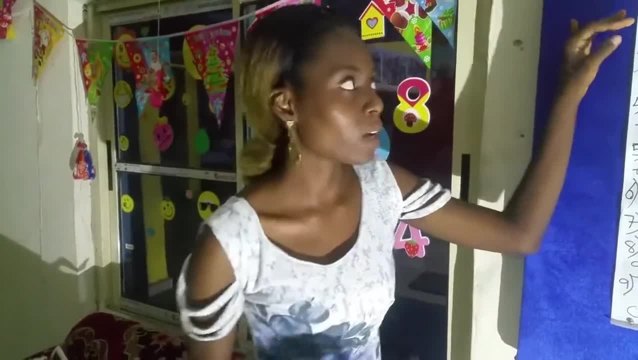 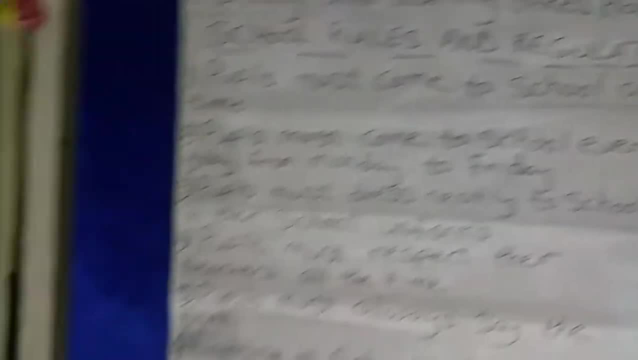 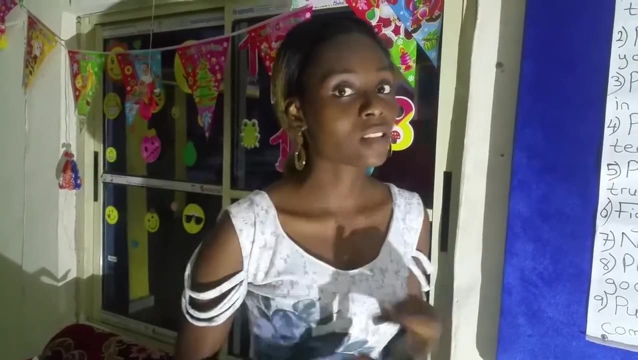 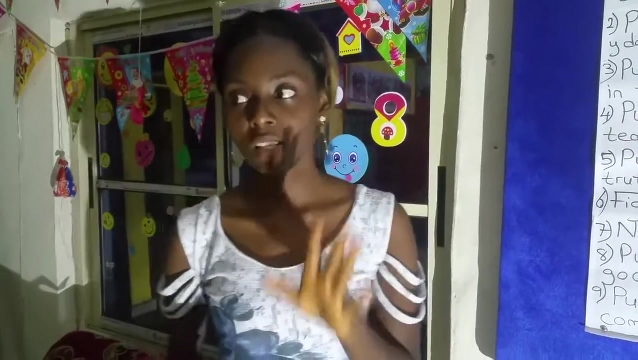 So if you want to go to school, you must go to school on time. And number two pupils must come to school every day, from Monday to Friday, From Mondays to Fridays. Okay, If you want to go to school as a student or as a pupil, you must go to school. Go on Monday, on Tuesday, on Wednesday, on Thursday and what? On Friday. If you skip school anyway, you'll be punished. So make sure you go to school for five days in the what In a week. 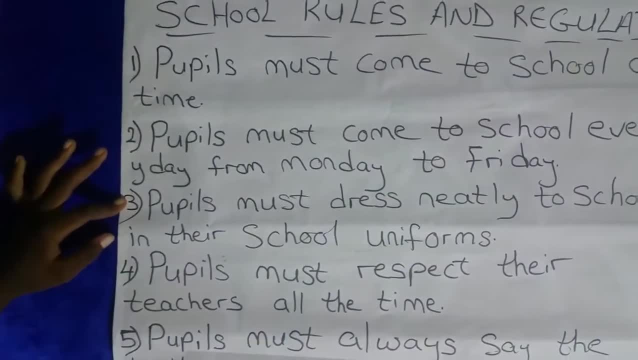 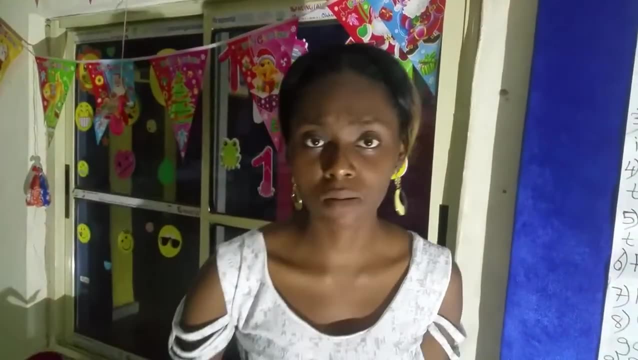 Now the third one: pupils must dress neatly to school in their school uniforms. If you want to go to school, you must put on your complete uniform. Do not wear slippers to school. You'll be punished. Wear your uniform, your top, your knickers or your skirts or your gown, Neatly well ironed Okay. 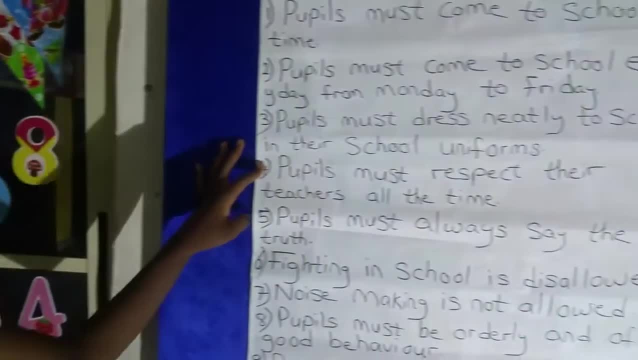 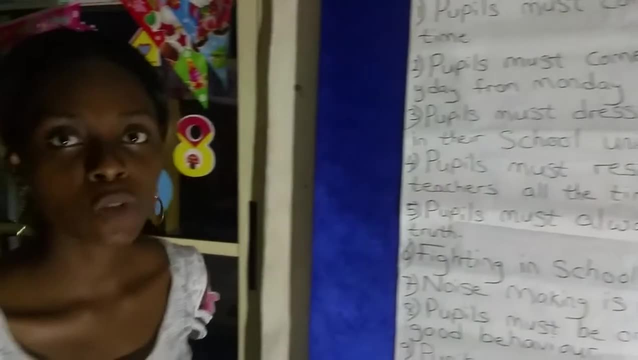 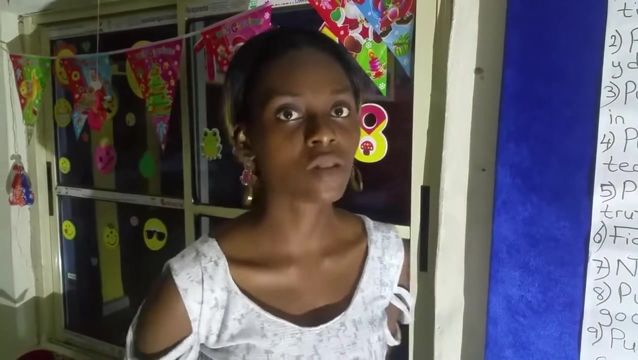 Now, what's the next one? Pupils must respect their teachers at all times. Pupils must respect their teachers at all times. Now, when you go to school, you meet your fellow students. you also meet teachers. Now, as a student or as a pupil, you must show your teachers respect. If you disrespect them, you'll be what Punished. You'll be what Punished. 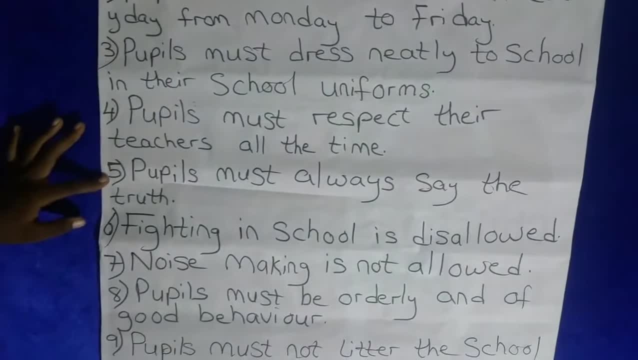 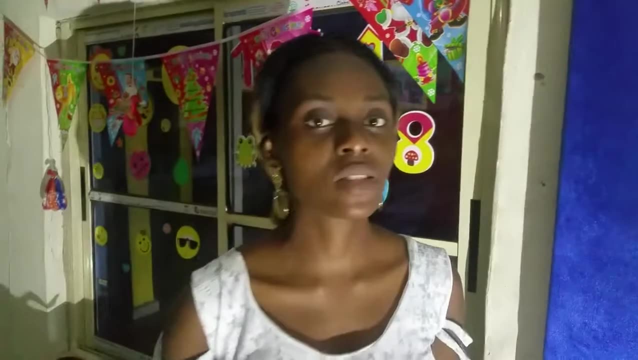 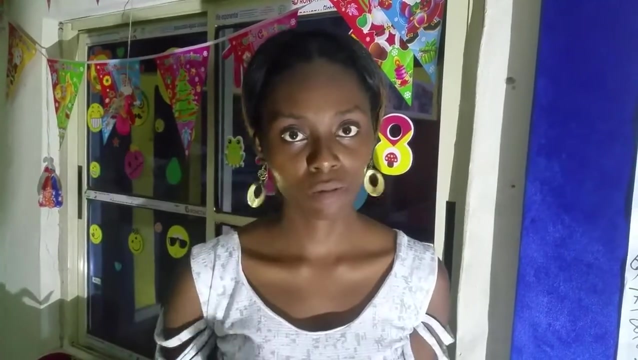 And the next one: pupils must always say the truth. Pupils must always say the truth. Do not tell lies. It's not good to tell lies. If you tell lies, you're committing a sin and you'll be punished. also, No matter what it is when you're asked, you must always say the truth. Don't tell lies. Even at home or in school. you must always say the truth. 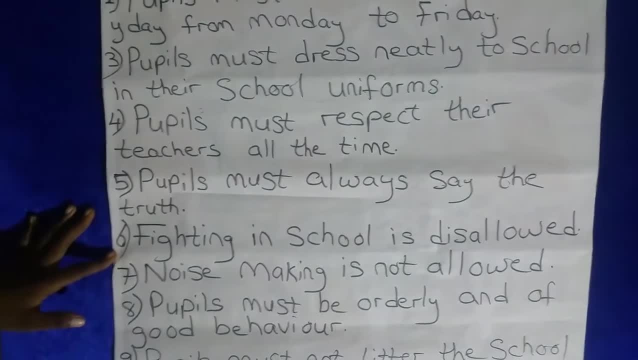 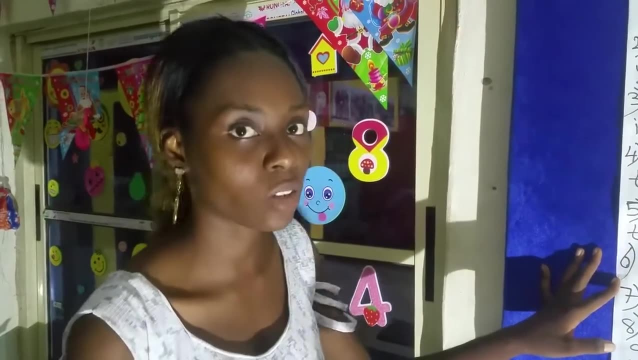 Now number six: fighting in the school is disallowed. When you go to school, do not fight. No matter what happens, do not fight. If they offend, you report to your class teacher. okay, Do not fight your fellow students. 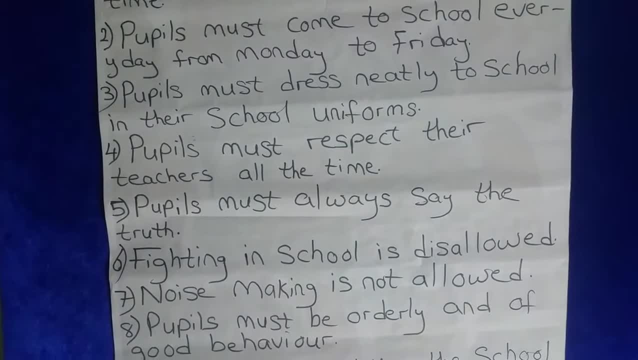 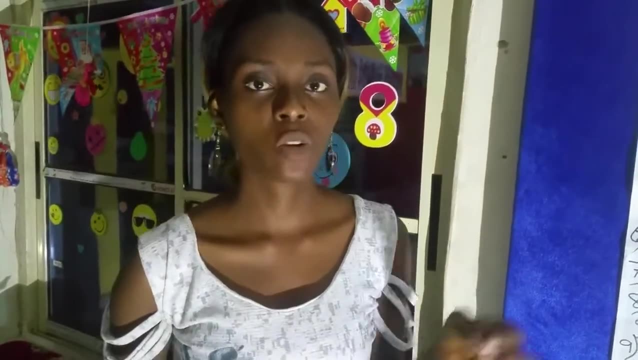 Number seven: noisemaking is not allowed. Noisemaking is not allowed. Do not make noise in the classroom. If you're in school, you should pay attention to what your teacher is saying. Do not make noise. Do not make noise. 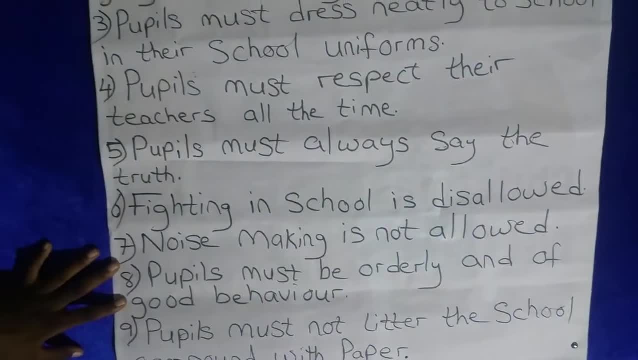 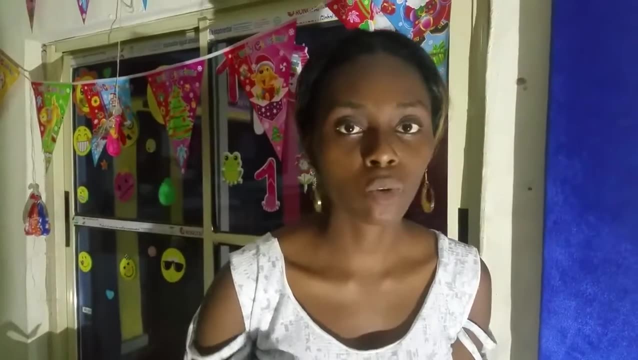 Number eight: pupils must be orderly and of good behavior. Pupils must be orderly and of good behavior. When you go to school, sit in your class carefully, Don't look for trouble, Don't steal someone's thing. Just pay attention and be a good student. Do you what? 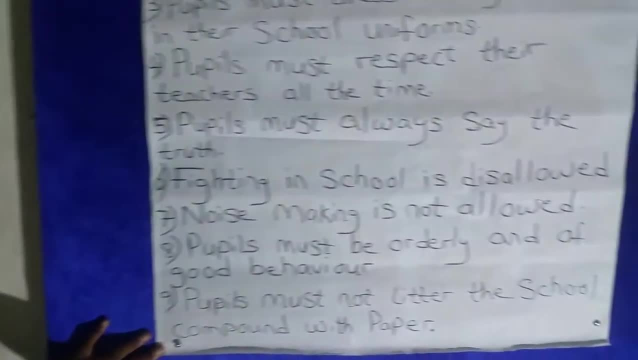 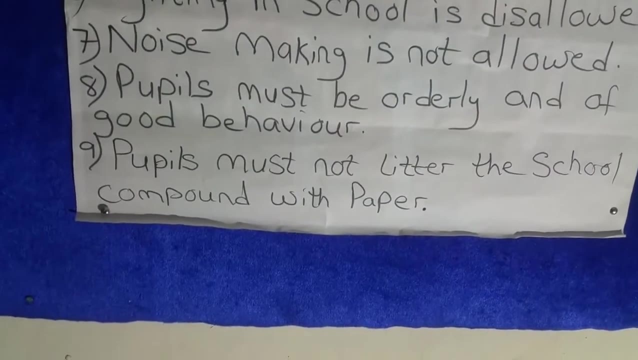 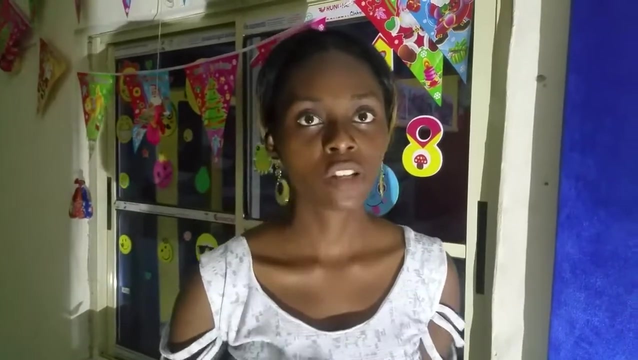 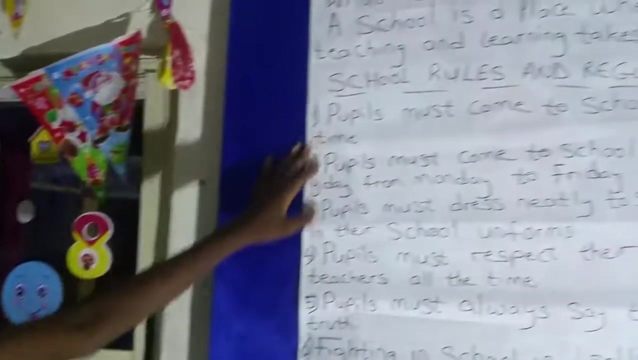 So you go home. Number nine: pupils must not litter the school compound with paper. There are waste bins everywhere around the school. There are trash cans. Now, once there's a paper you want to throw away, throw it in the waste bin or the trash can. Don't litter the school environment. If you are caught doing so, you'll be punished. So these are the rules and regulations you have to keep as a pupil. If you want to go to school, you must learn how to adhere to all of these rules and regulations. If you fail any of them, you will be punished. 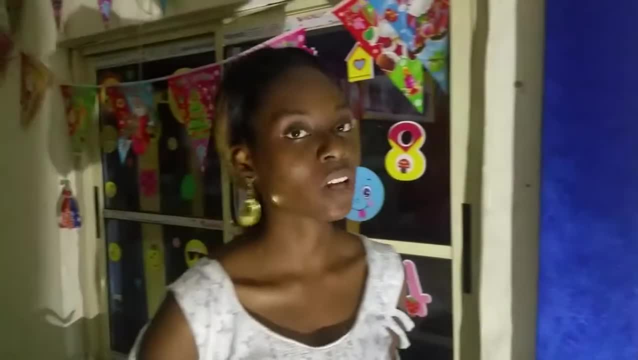 So make sure you know the different rules and regulations And don't forget them. Be good at all times. Bye. 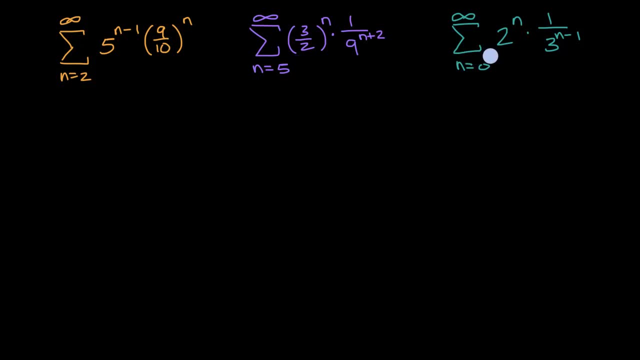 So here we have three different series, and what I would like you to do is pause this video and think about whether each of them converges or diverges. All right, now, let's work on this together. So, just as a refresher, converge means 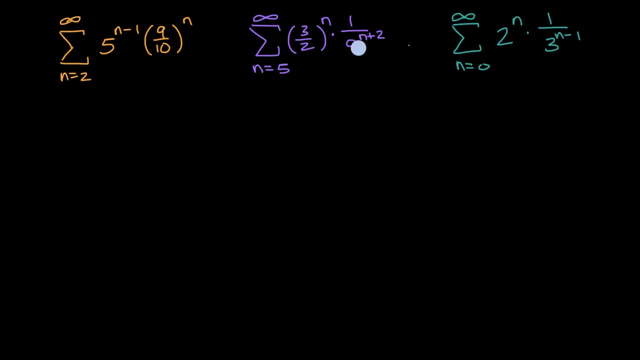 that, even though you're summing up an infinite number of terms, in all of these cases, if they converge, that means you actually get a finite value for that infinite sum or that infinite number of terms being summed up, which I always find somewhat amazing. 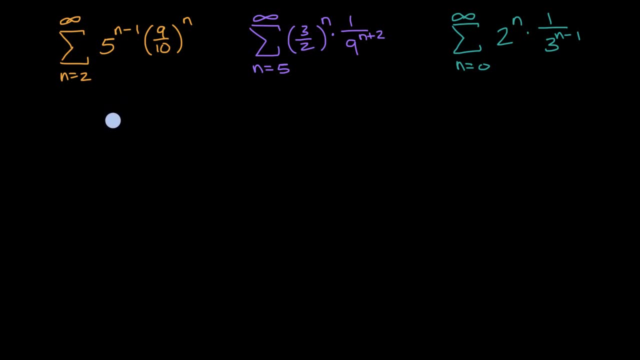 and diverging means that you're not going to get an actual finite value for the sum of all of the infinite terms. So how do we think about that? Well, we already know something about geometric series, and these look kinda like geometric series. 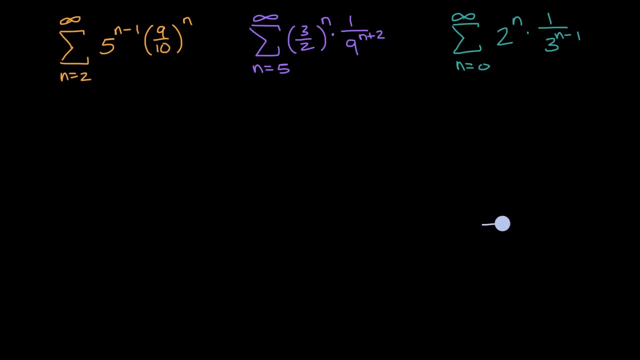 so let's just remind ourselves what we already know. We know that a geometric series, the standard way of writing it is we're starting, n equals. typically you'll often see n is equal to zero, but let's say we're starting at some constant. 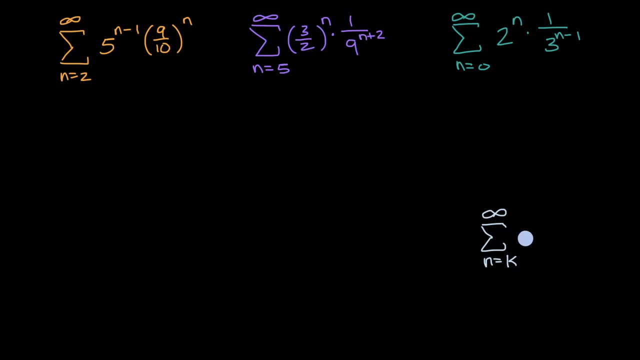 and then you're going to have- you're going to go to infinity- of a times r to the n, where r is our common ratio. We've talked about that in depth in other videos. We know this is the standard way to write a geometric series.